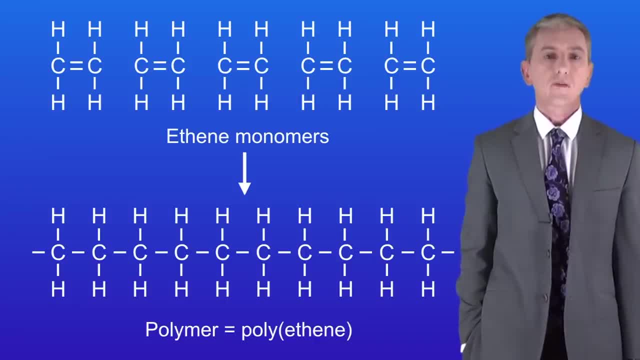 called polyethene. Now there are several points about this that you need to learn. Firstly, the monomer has a double carbon to carbon covalent bond. We can see these here. However, the polymer contains single carbon to carbon covalent bonds, and here they are. 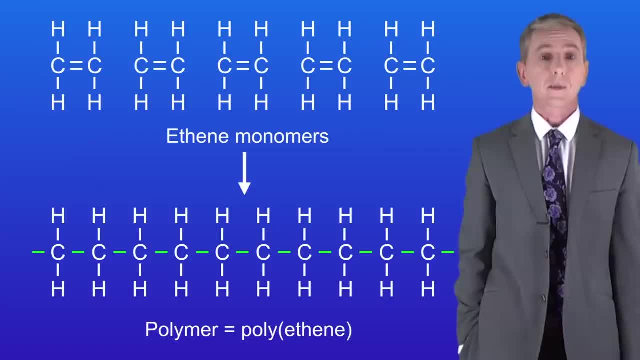 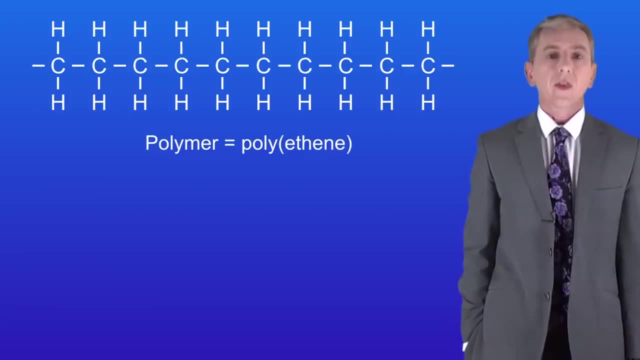 Remember that, because these bonds are covalent, they're extremely strong. Students often ask what happens at the ends of the polymer molecule. You don't need to know that and you won't be asked that in the exam. Now, there is one problem with drawing a polymer such as this, and that is that. 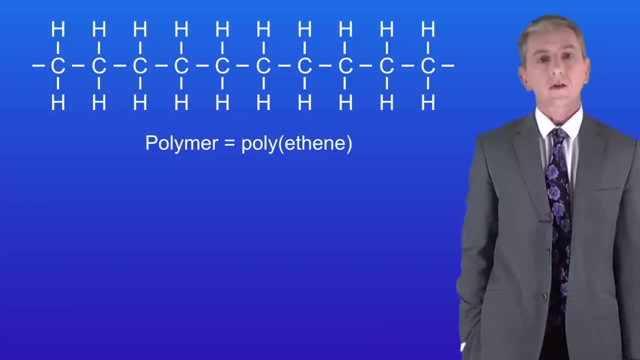 there are lots of atoms and covalent bonds to draw, So scientists usually draw it in a short hand way like this. This is called the repeating unit. There are three important details about the repeating unit that you need to learn. Firstly, remember that it shows a single carbon. 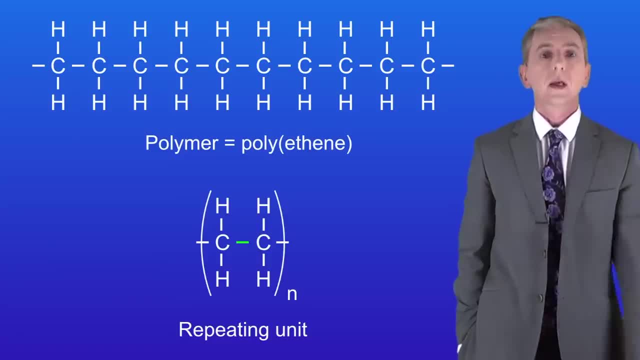 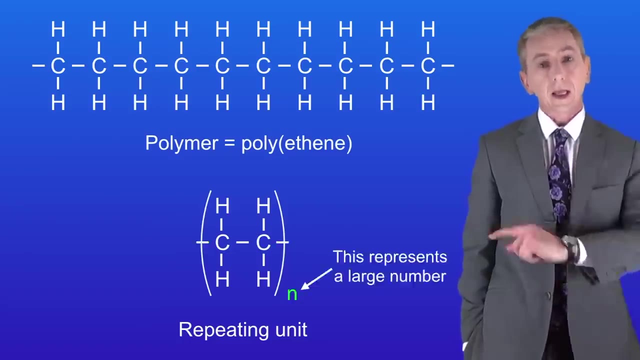 to carbon covalent bond, and we can see that here. Secondly, the covalent bonds on either side have to extend out of the brackets like this. This tells us that the polymer molecule extends out in both directions. Lastly, the little n here. 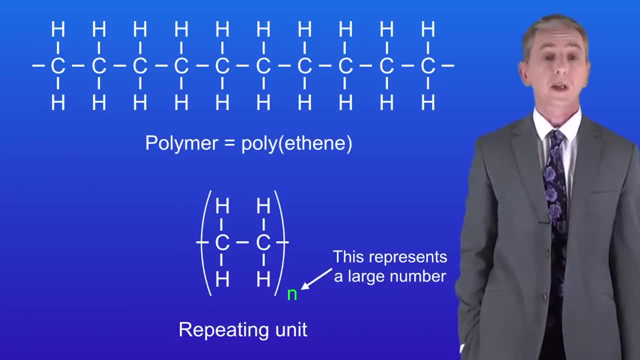 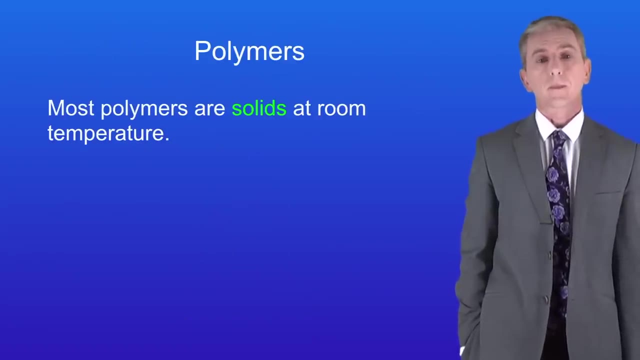 tells us that the polymer contains a very large number of repeating units. joined together, N just represents a large number. Okay, we're going to move on now and look at a key property of polymers which you need to be able to explain. Most polymers are solids at room temperature. That's because the 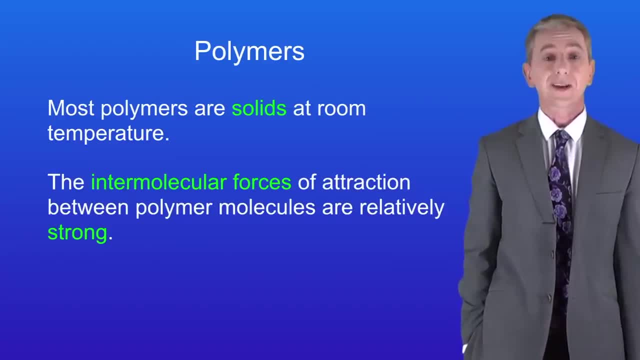 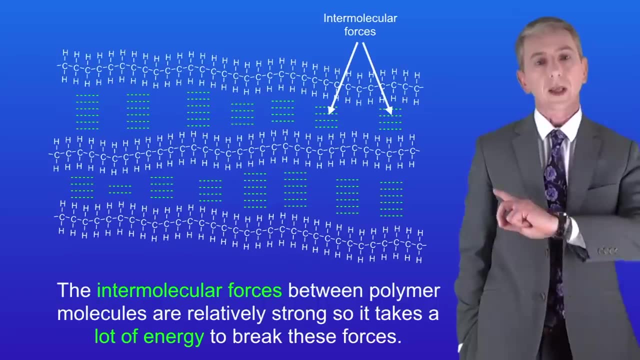 intermolecular forces of attraction between polymer molecules are relatively strong. Now this sounds a bit tricky, but it's quite straightforward. I'm showing you polymer molecules here. As you can see, we've got a lot of intermolecular forces of attraction acting between the polymer molecules. It takes a lot of. 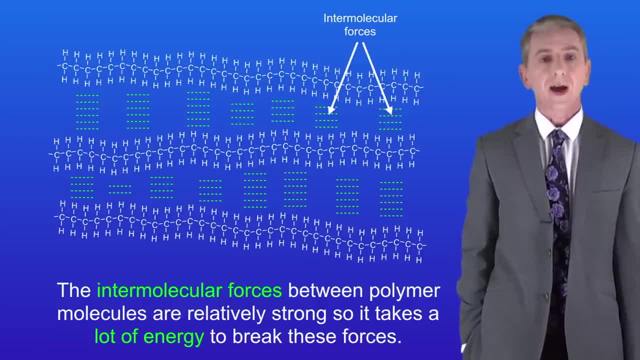 energy to break these forces. so that means that polymers have a high melting point. Most polymers are solids at room temperature. Remember, you'll find plenty of questions on polymers in my revision workbook and you can get that by clicking on the link above. And if you're doing triple chemistry you're going to. 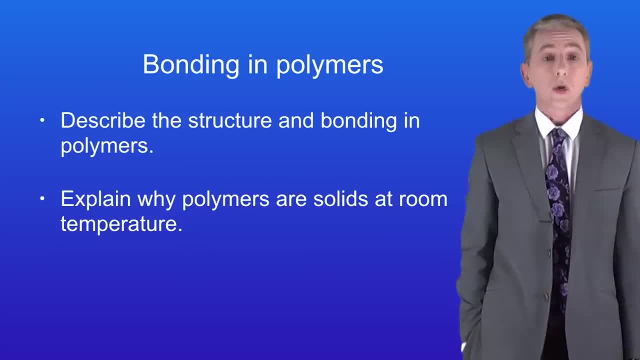 be seeing a lot more about polymers in later videos. Okay, so hopefully now you should be able to describe the structure and the bonding and polymers. You should then be able to explain why polymers are solids at room temperature.